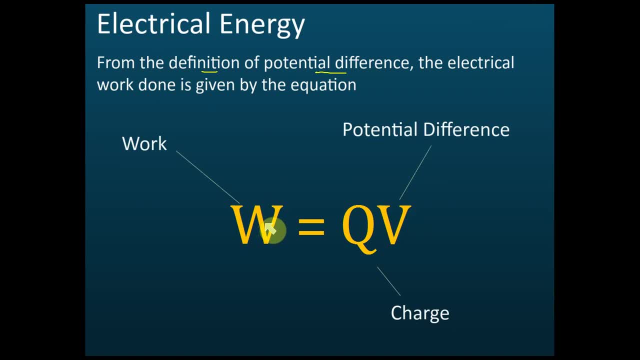 electrical work, dance, and in form four, we have learned that the amount of work done is equal to the amount of energy used to do the work. okay, because we need to, we need energy to do work, we need energy to do work, and how much work done is equal to how much energy used to do work. so therefore, uh, we can write our 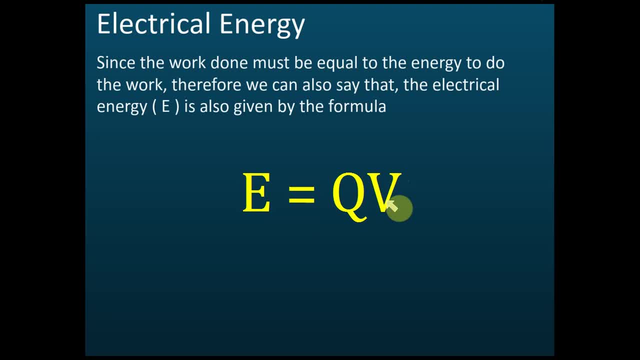 this uh formula just now it's w equals to qv. okay, then we can also write e equal to qv, because the amount of work done and the amount of energy used is the same, so e equal to qv. so work then must be equal to the energy to do the work. so then the formula become e equal to qv and uh. this is the. 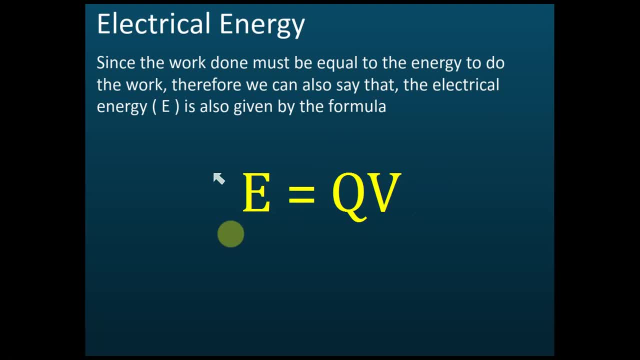 formula: okay, this is the formula that we are going to use to find electrical energy. electrical energy sometimes the questions they don't. they won't give you q the charge. okay, because it's very hard for us to measure charge. so we can use a wood meter to measure a voltage and we can use 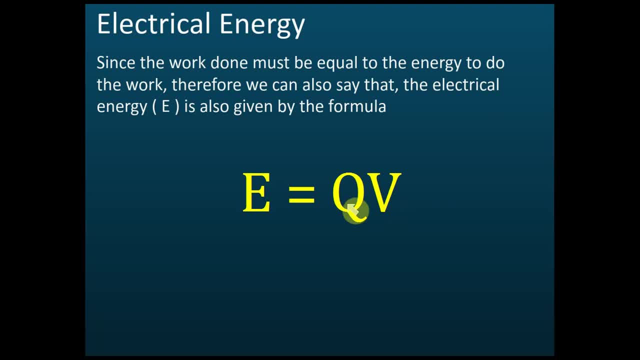 emitter to measure current. okay, but it's very hard for you for us to measure charge uh. then therefore, we can uh do some modifications to this formula. so we have learned that uh charge q equal to i t. this is from the definitions of current. current is the rate of charge flow i. 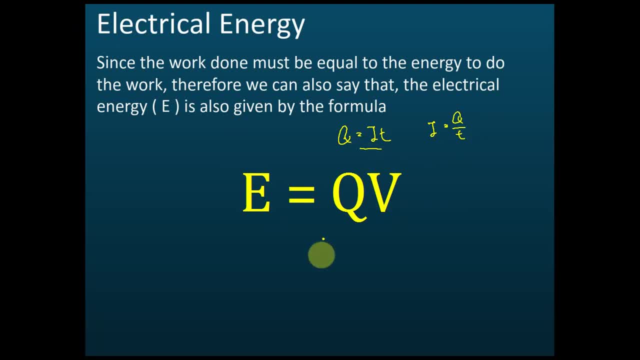 equals to q over t. therefore q equal to i t. so if q equal to i t, then this formula will become itv or vit, vit. so you need to remember: uh, electrical energy is equal to qv or vit. it is actually is equal to q because q with it. so these two formulas. 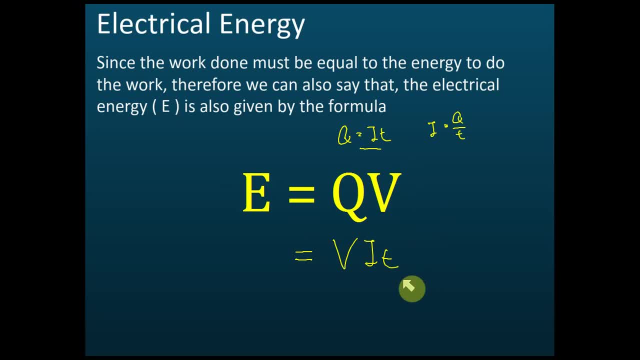 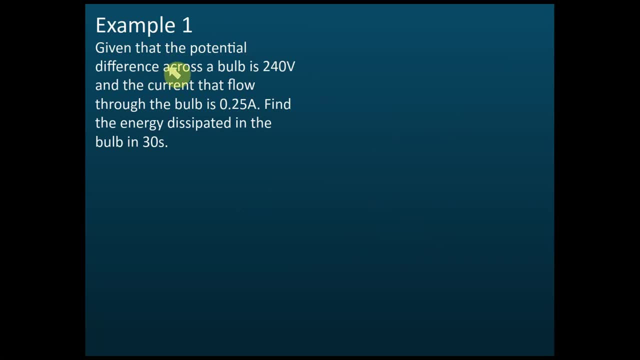 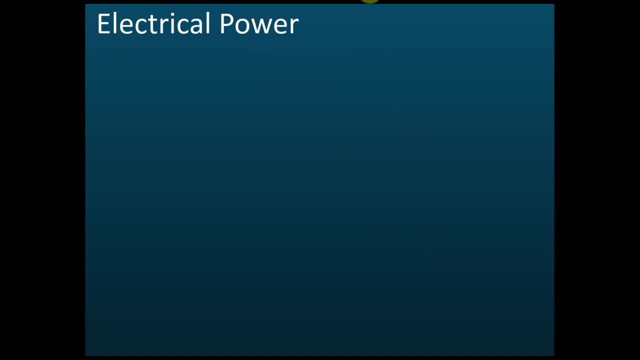 formula. there should be no problem for you, okay. next, electrical power. yeah, electrical power. uh, in form four we have learned power. in form four, you have learned power under force and motions. power is defined as a rates- rates of work done or rates of energy supply- rates of work done or rates of energy supply- and the unit is 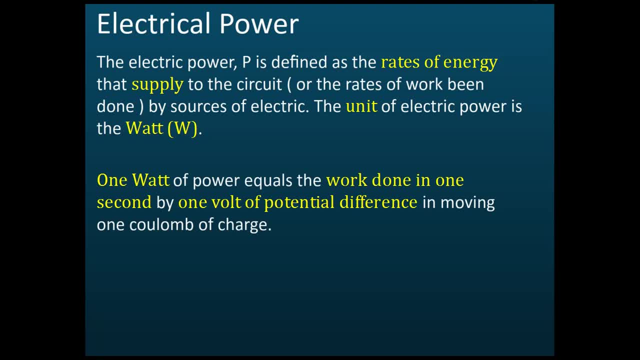 watt. so from the definitions uh, from the definitions uh, power is given by the formula p equal to w over t, right rates of energy supply, uh, p equals to the energy, then should be e okay, e over t okay. if, if it's a rate of work done, then p equals to w over t. yeah, and the unit is watt. 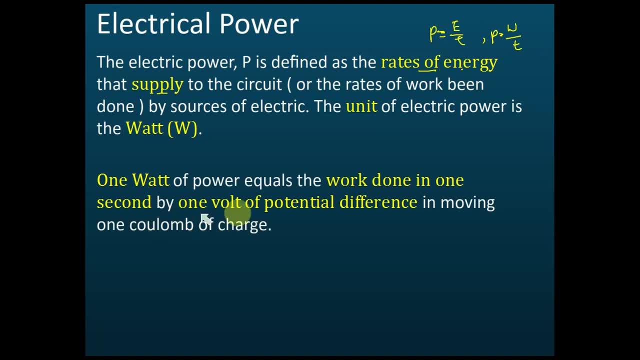 one watt means uh, work done in one second, by one word of potential difference, to move the one columns of charge. so that is uh one watt. this that is electrical power. electrical power one watt means work done in one second, by one word of potential difference, to move one columns of. 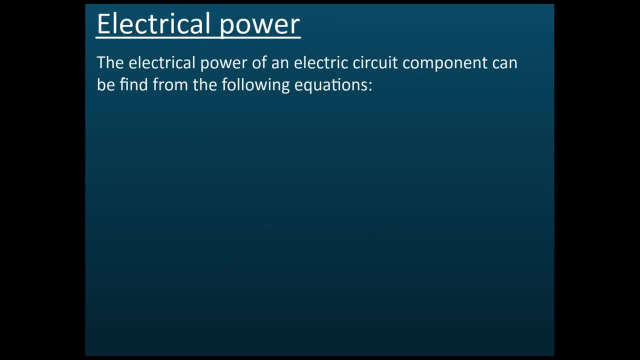 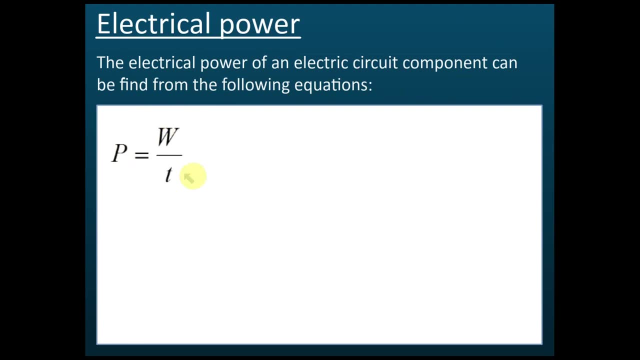 charge. so the equations uh, from the definitions of power, p equal to w over t right, p equal to w over t yeah, or p equal to e over t, p equal to w over t or p equal to e over e over t yeah, just now we have learned that uh e equal to qv right, electrical energy equates. 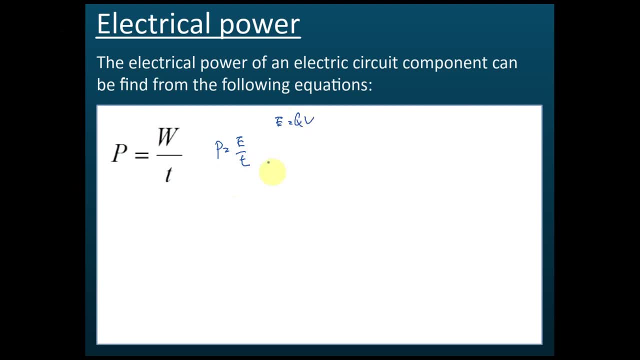 to qv. so from e to q video. then p equals to qv, qv over t. just now we also learned that the current i equal to q over t. right, because current is the rate of charge flow, how fast the charge flow. i equal to q over t. so this q over t is equal to current. so then 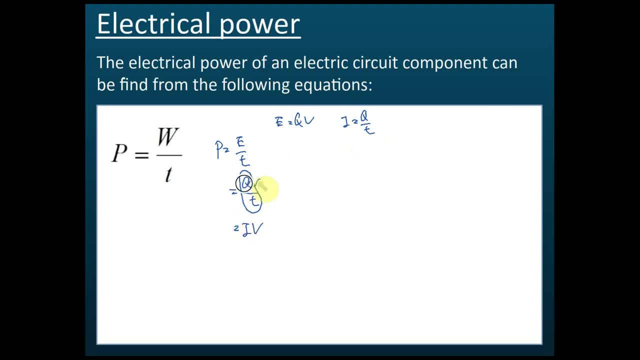 the equation become: i. v should be q v, sorry, it should be. should be e over t. but uh, e equal to q v and q over t is equal to current. so, uh, the power. okay, the power uh can be calculated by using this formula: p equal to iv. now, this is uh the general formula. this is a general formula. 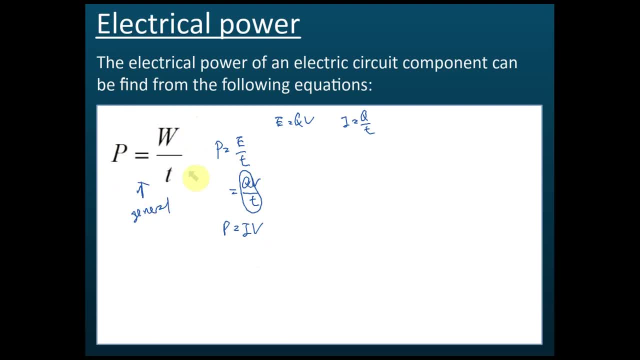 general formula for power. you can use this to do all the calculations related to power. this one is only for electrical power. this is only for electrical power, so p equals iv. from ohm's law we also learned that v equals ir. right, we got ir. uh, so this p 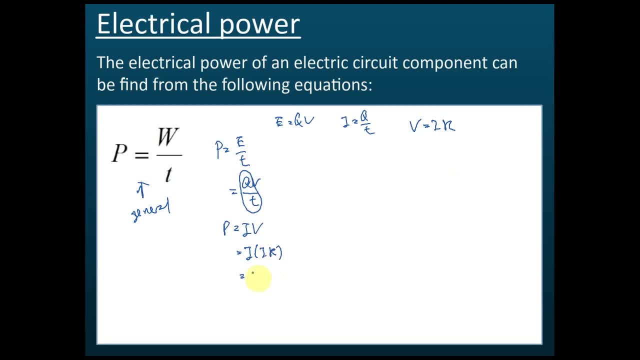 equals to i. this v equals ir. so therefore, is equals to i square r. so we have p equals to iv and p equals to i square r. okay, so it depends on the questions, whether the qu to see whether the questions give you currents voltage or a current resistance. okay now, from this v equal to ir, we 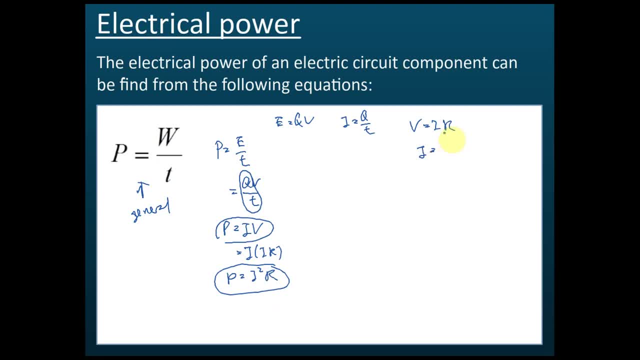 also learned that we can rewrite this. then it become: i equals to. we move r to another side, so it become v over r, so i equals v over r. now let's substitute this i equals v over r into these equations: uh, so then the p equals to the i become v over r. and then times v, times this v, uh, then it become v square. 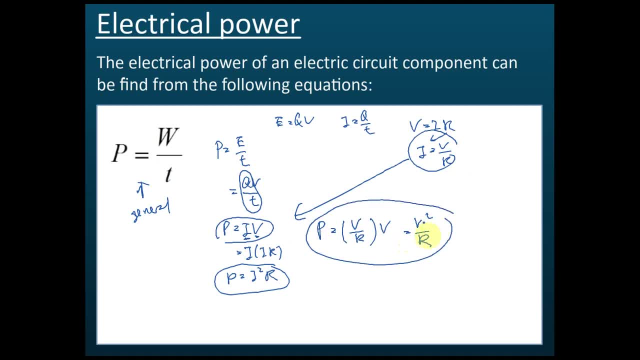 over r. uh, this is the third equation for power. so we have uh three formula for electrical power: p equals iv, p equals i square r and p equals to v square over r. these three are electrical power. this is a general formula for power, but if you don't know how to get this, how to derive this? 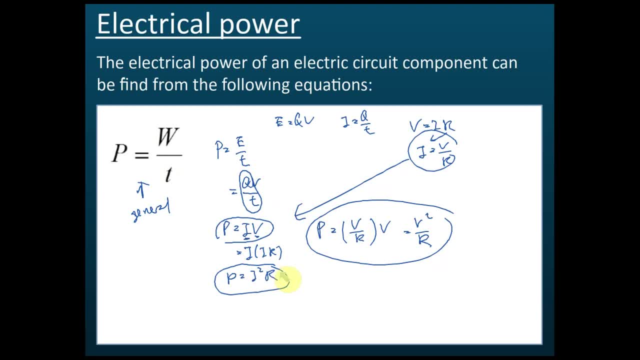 it's okay. how to derive this, how to get this formula, is not important. what's important is that you must remember or memorize this formula. so let's erase this. so we have p equals iv, p equals i square r and p equals to v square over r. so in this formula, p is power, w is work done, t is time i. 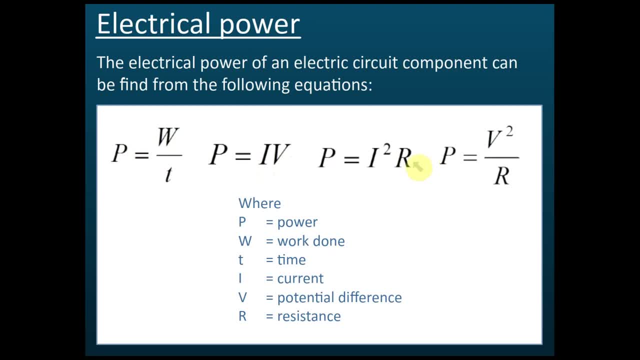 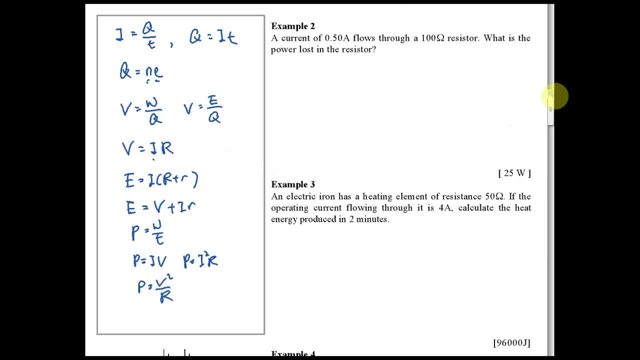 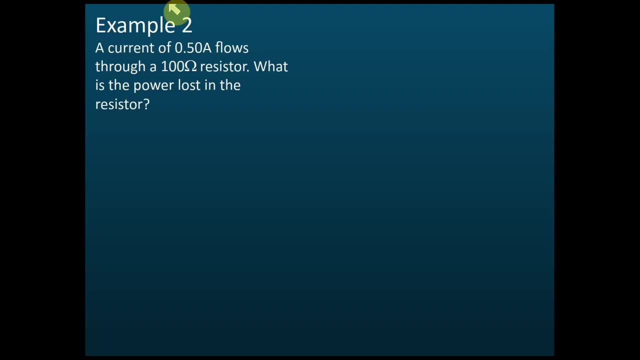 v is voltage and r is the resistance. so make sure that you remember or memorize all of this. okay, all of this formula. so these are the uh formula or equations that we have learned so far in this chapter. okay, example two: occurrence of 0.5 ampere flows through a 100 ohm resistor. what is the power? 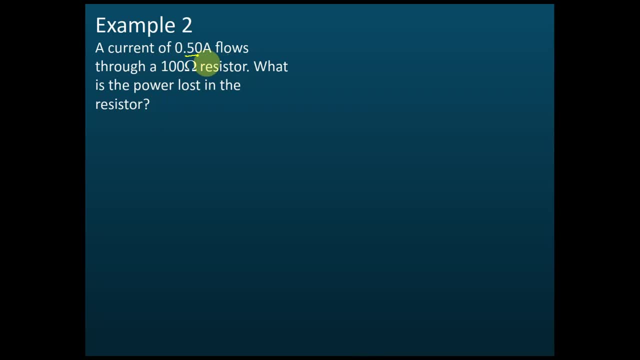 loss in the resistor. okay, so this answer: okay, so the current 0.5 ampere resistance 100 ohm. so, uh, so, since we have i and r, so then we use this formula: p equals to i square r, so substitute this two number into the formula, then you get p equal to 25 watt. okay, example three: 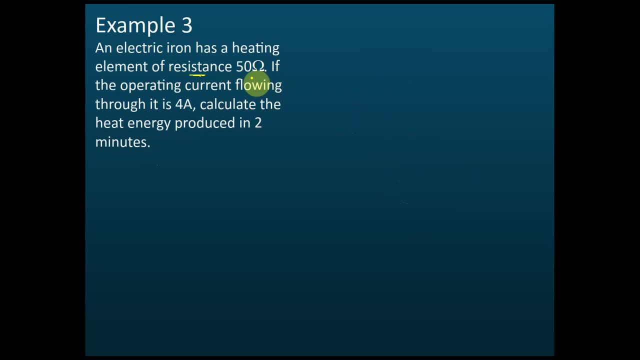 calculate the heat energy produced in two minutes. so we have here the quiero. so so the answer is uh 96 000, 96 000 joule. okay, so you see, uh, uh. at the very beginnings i list down all the informations that i have: uh r equals to 50 ohm, and then i equals to uh four ampere. okay, 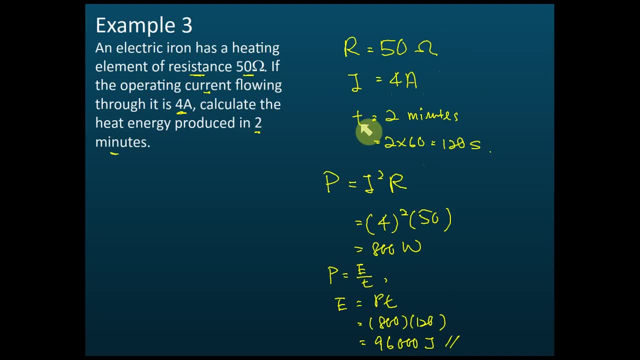 four ampere and uh, uh t. is t equal to two minutes, two minutes of? i can use this: p equals to i square r to find my power. okay, which is equal to uh 800 watt, okay, 800 watt. and then start to find the heat energy. to find the heat energy, i can use the formulas of power p equal to w over t or p equal. 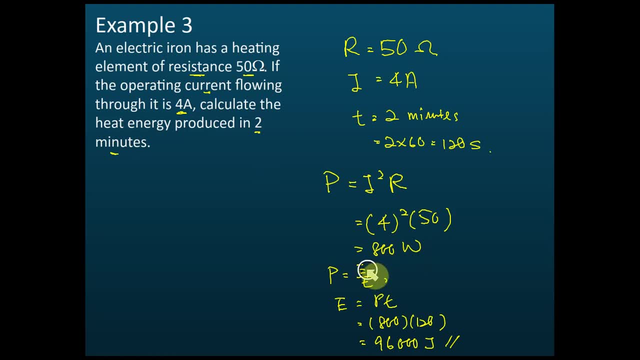 to e over t, and e is the energy, e is energy, so p equal to e over t. uh, therefore e equal to pt. okay, pt, and here i have my power, 800 watt, so i substitute this into p here. okay, and the time taken is 120.